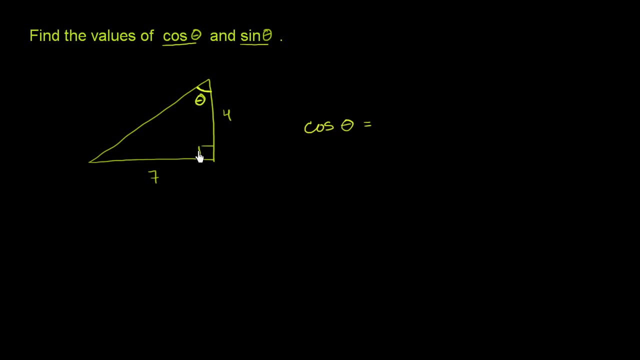 theta is this angle right over here, and it is indeed a right triangle. So I'll give you a few seconds to think about that. Well, to answer this, you just have to remember the definitions of the trig functions, And to help us there, we'll use the mnemonic SOH-CAH-TOA. 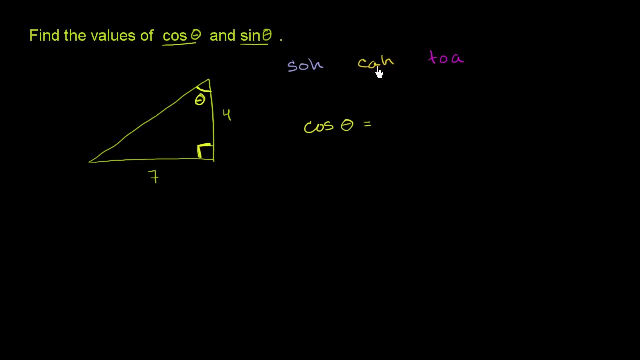 And the part of SOH-CAH-TOA that relates to cosine is the CAH part. This defines sine. That's why we have the s. This defines cosine. That's what starts with the c. This defines tangent. That's why it starts with a t. 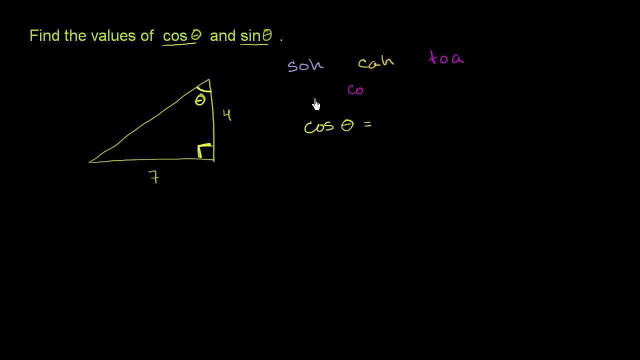 So if you look at CAH, it says that cosine. let me do it next. It's that same color. It says that cosine of an angle is equal to the adjacent side over the hypotenuse. So in our example here, what is the adjacent side? 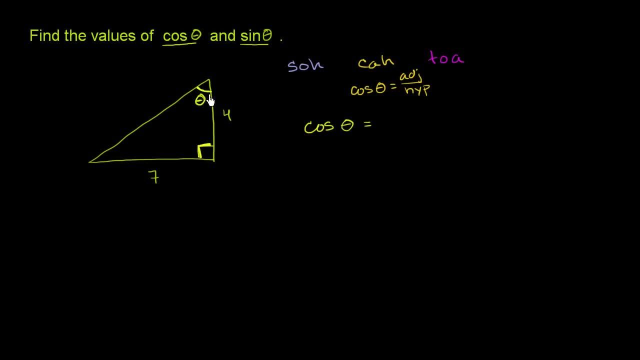 Well, if we look at it, it's the side that's next to it, that is not the hypotenuse. This side is next to it and it's not the hypotenuse. This side up here is next to our angle. 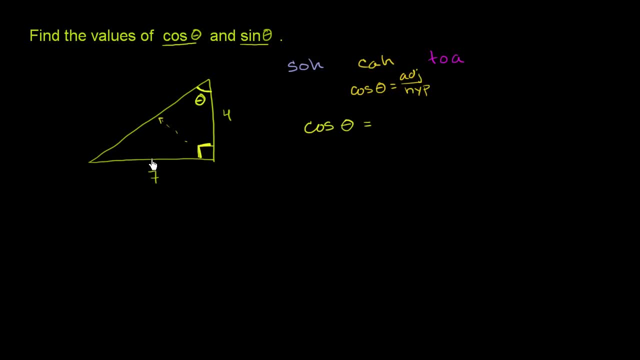 but it is the hypotenuse. It's the one that's opposite the right angle. So this is the hypotenuse up here. This is if we're looking at angle theta. this is the adjacent side. And while we're at it, if we want, 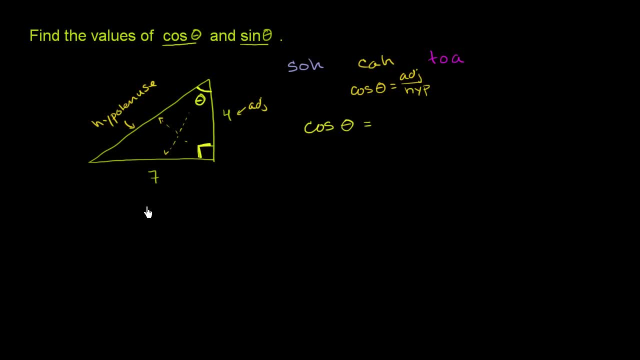 to think about the opposite side. we don't have to deal with it for cosine, but it doesn't hurt to label it right now. That is the opposite And this is relative to angle theta. So with that out of the way, we said cosine of theta. 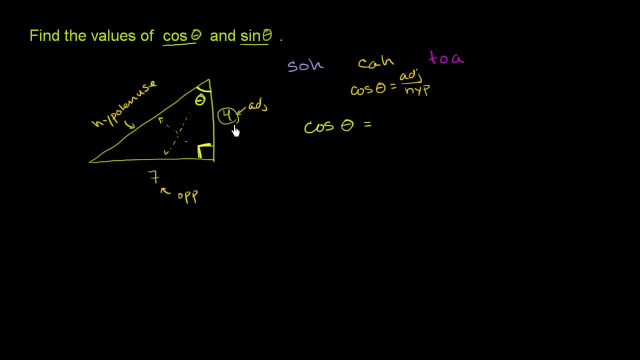 is equal to adjacent over hypotenuse. Adjacent has length 4.. What is the hypotenuse? Well, we know what side is the hypotenuse, but they haven't given us the length yet. But we can figure it out using the Pythagorean theorem. 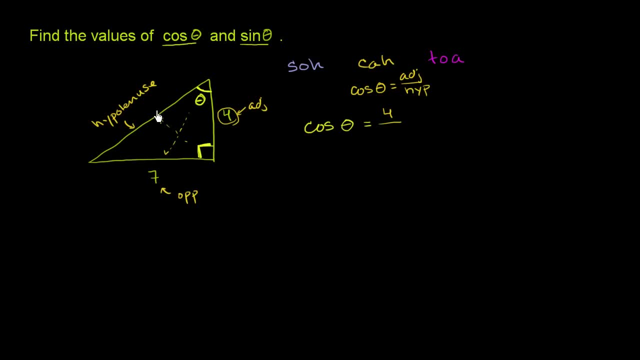 We have two sides of a right triangle. We can always figure out the third side. We know that the sum of the squares of the two shorter sides will be equal to the square of the hypotenuse. So we have 4 squared Plus 7 squared is going to be equal to.